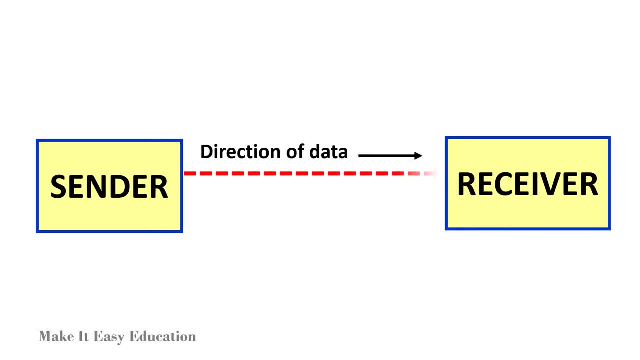 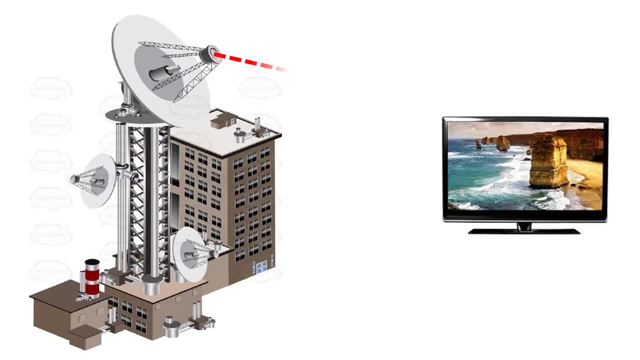 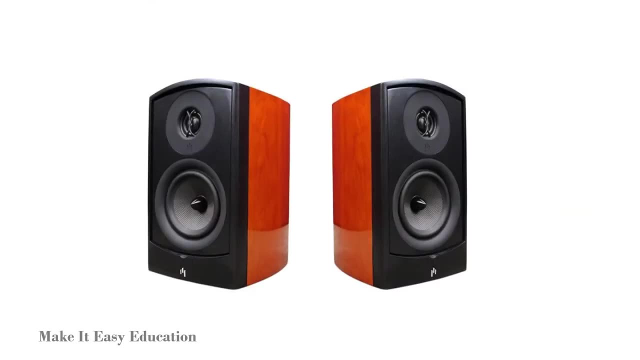 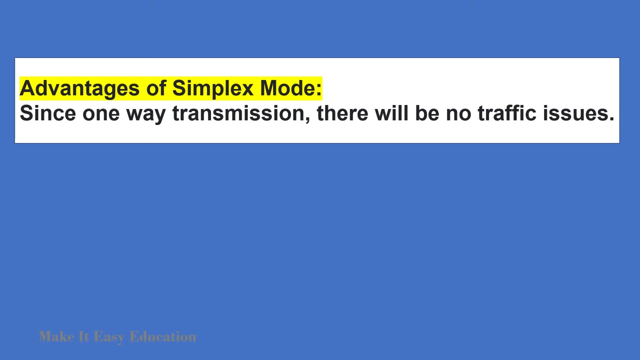 that is, communication is unidirectional. We cannot send a message back to the sender. Examples of simplex mode are television broadcasting, keyboard sending data to the monitor and music or any sound coming from the loudspeakers. Advantages of simplex mode: Since one-way transmission, there will be no traffic issues. 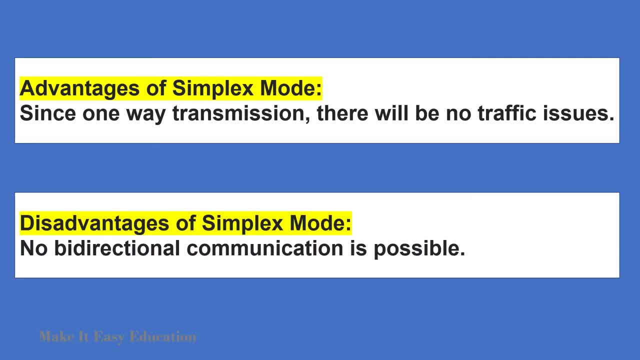 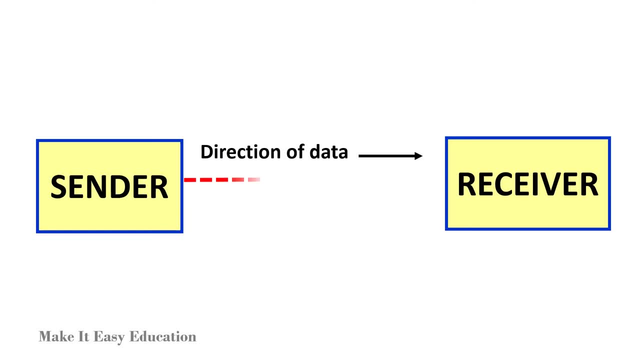 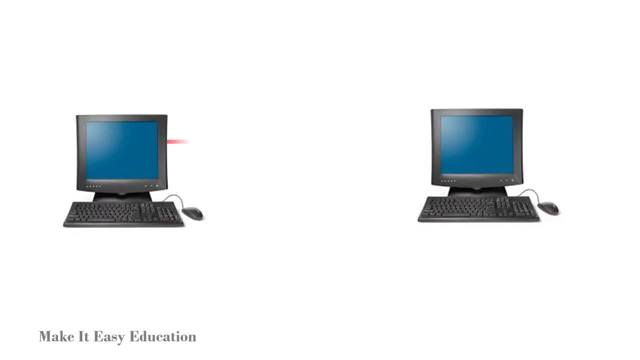 Disadvantages of simplex mode: No bidirectional communication is possible. Half duplex In half duplex mode transmission: data can be transmitted in both directions, but not at the same time. If one device is sending data, then the other device cannot send data until it receives the data. 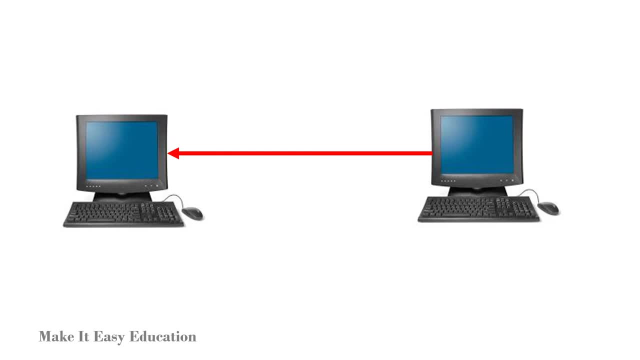 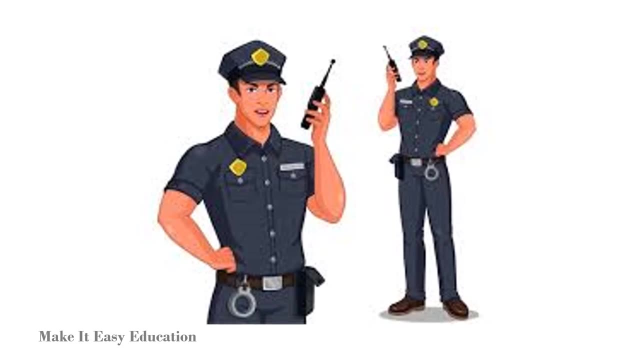 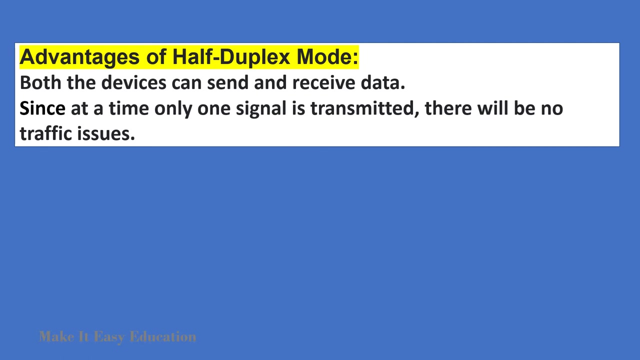 Communication is not simultaneous. Example of half duplex is a walkie-talkie in which message is sent in both the directions, but not at the same time. Advantages of half duplex mode: Both the devices can send and receive data. Since at a time only one signal is transmitted, there will be no traffic issues. 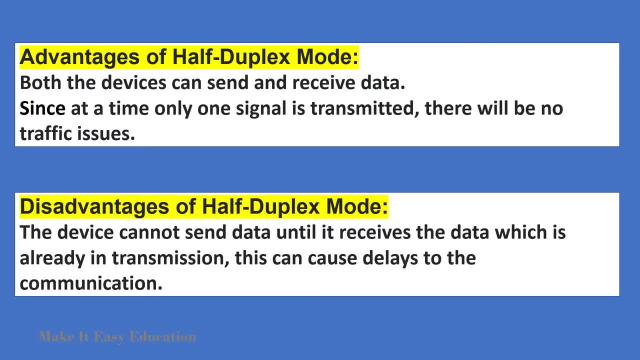 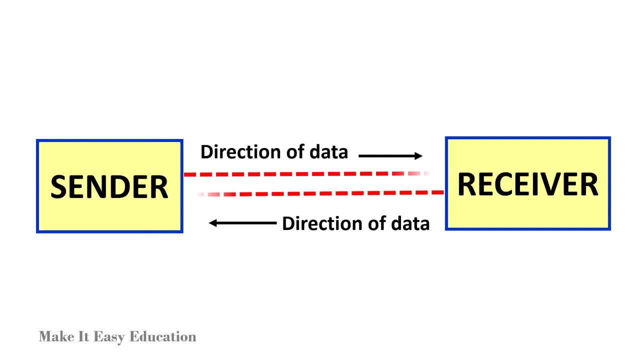 Disadvantages of half duplex mode: The device cannot send data until it receives the data. This can cause delays to the communication. Full duplex. In full duplex mode, both the connected devices can send and receive data simultaneously. Transmission is bidirectional at the same time. 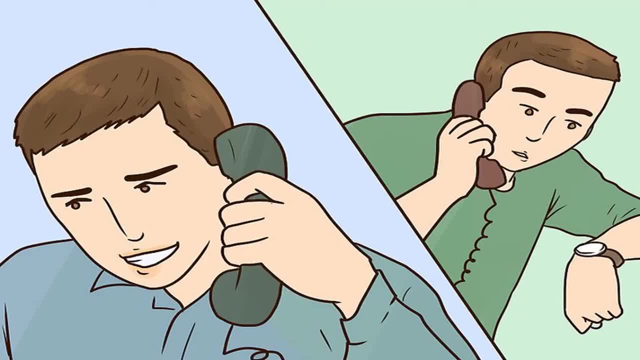 Example of full duplex is a telephone network in which there is communication between two persons by a telephone line using which both can talk. Disadvantages of full duplex mode: The device can talk and listen at the same time. Advantages of full duplex mode: No delays in communication. 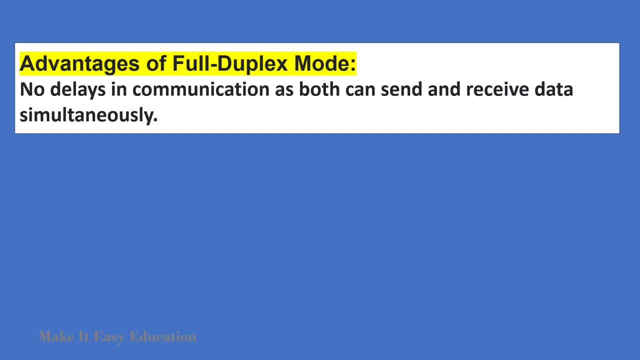 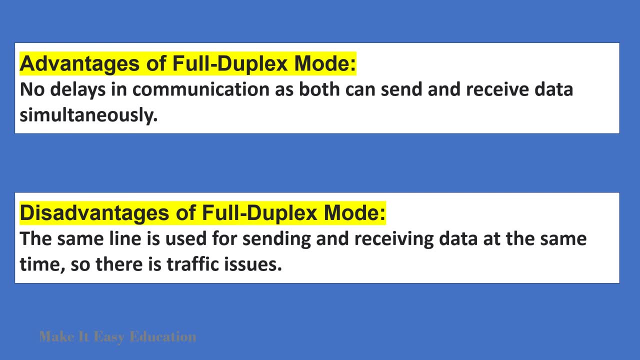 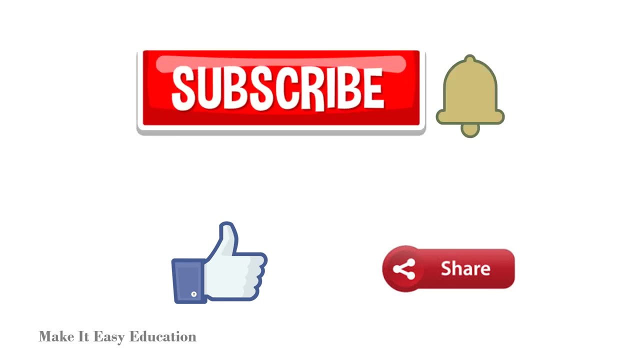 as both can send and receive data simultaneously. Disadvantages of full duplex mode. The same line is used for sending and receiving data at the same time, so there is traffic issues. Every week you will be notified by a new video, So don't forget to subscribe and click the. 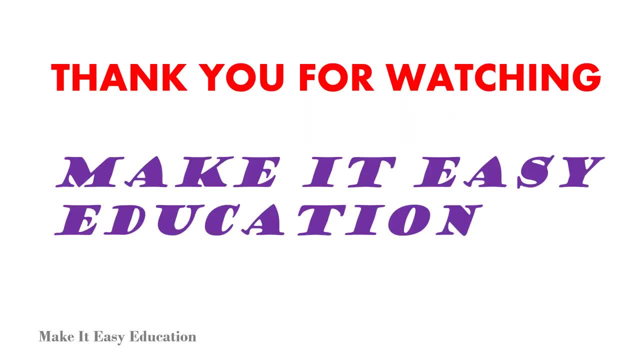 notification bell. Thank you for watching. make it easy education.